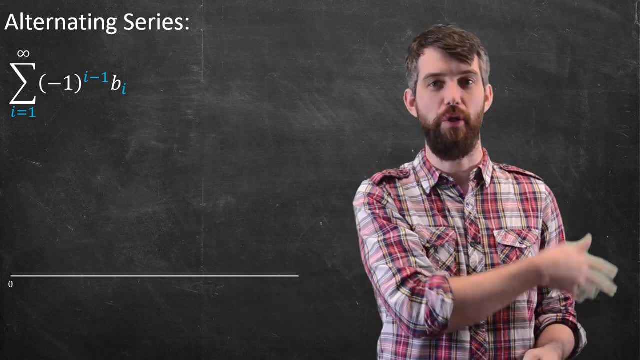 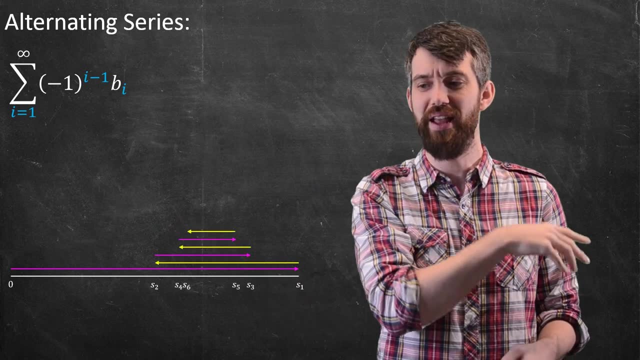 this sort of back and forth behavior where the s1 was going to go all the way out and then the s2 was going to go back in, and then the s3 was going to go out and s4 back in and s5 out and s6 and s7. 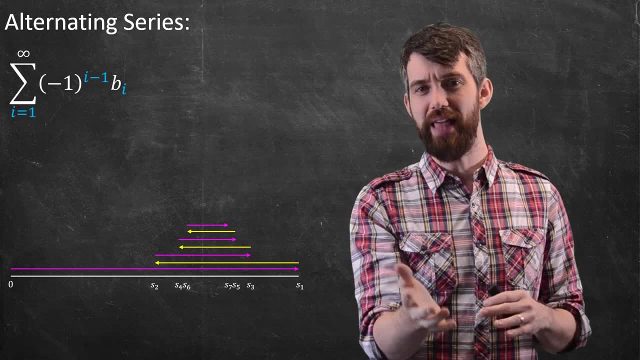 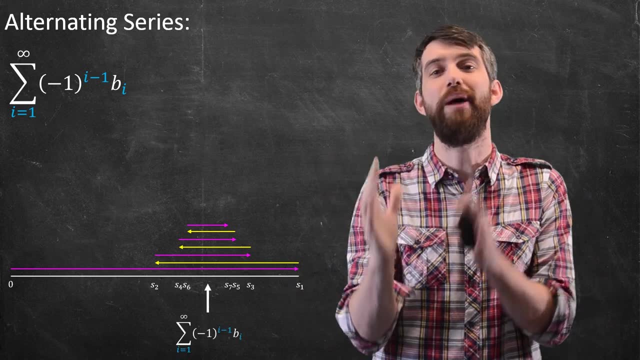 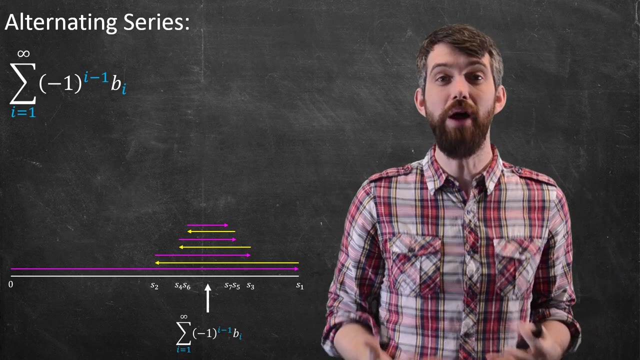 and it just could back and forth and back and forth like that, And then we concluded that the actual sum of the series was going to converge in this kind of case and it was somewhere in the middle, squashed between this alternating behavior. Now, let me suppose I've done that and I want to. 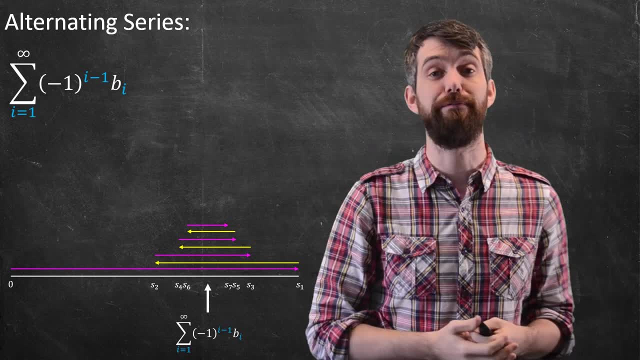 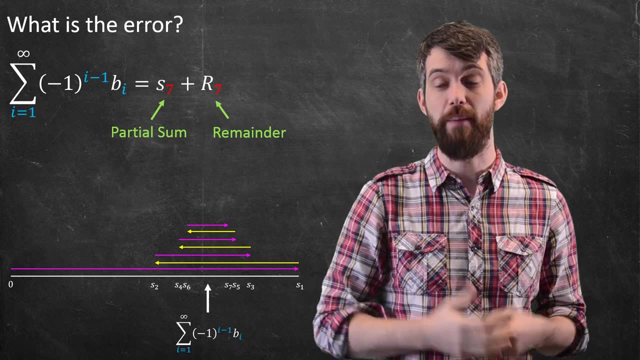 go and try to estimate this by perhaps only these first seven terms. That is, I have this series and I want to estimate this by perhaps only these first seven terms. That is, I have this series and I want to want to go and write it as the sum of a partial sum- S7, and some remainder, some error term- R7. 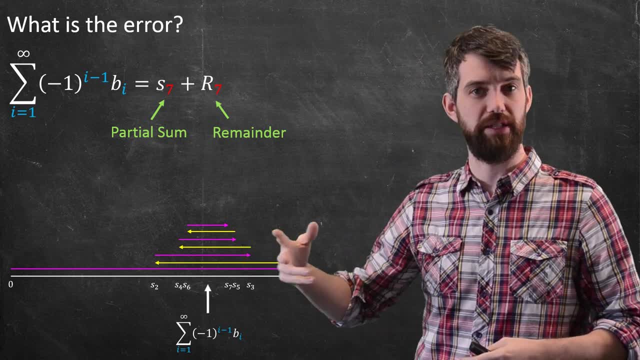 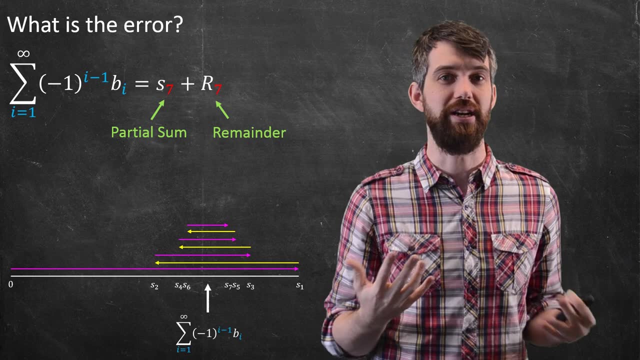 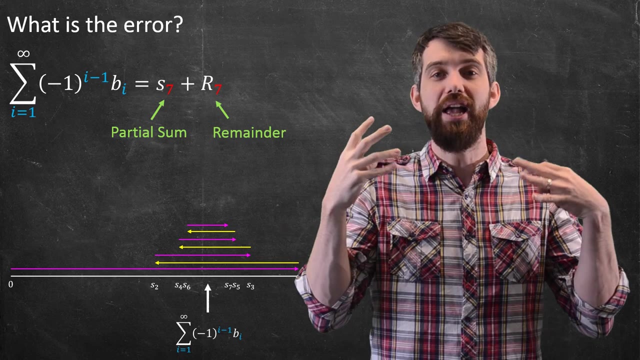 Now I don't know where exactly this sum is. It could be anywhere in this particular region, But let me try to approximate it by, say, the S7.. So the question is: how good is this error? If I take this R7, is it a small number? Is it a big number? How can I control how bad my estimate? 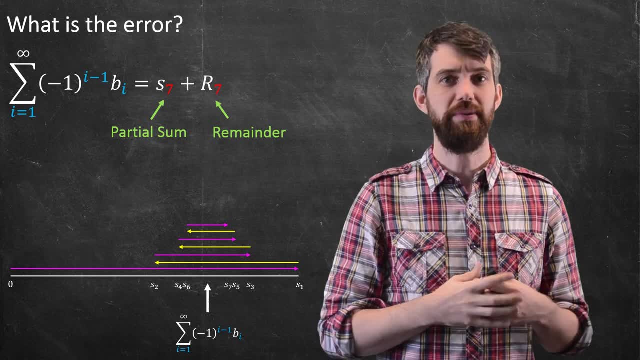 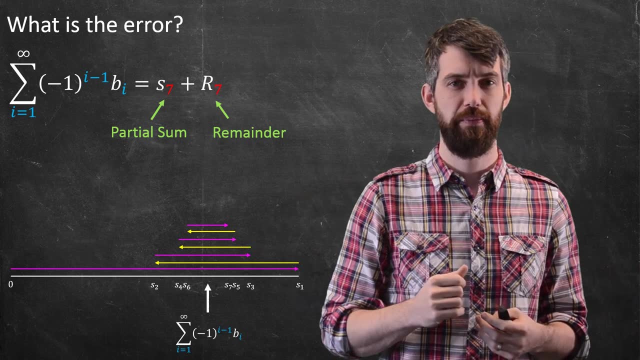 of only taking the first seven terms is going to be Now to think about what this remainder could be. we're currently at the S7. And imagine we want to go from the S7 out to an S8. Well, after we went, 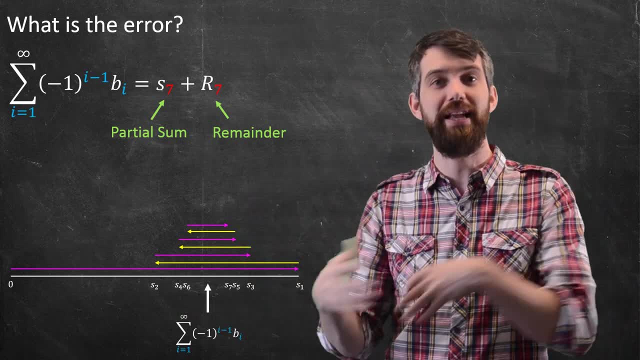 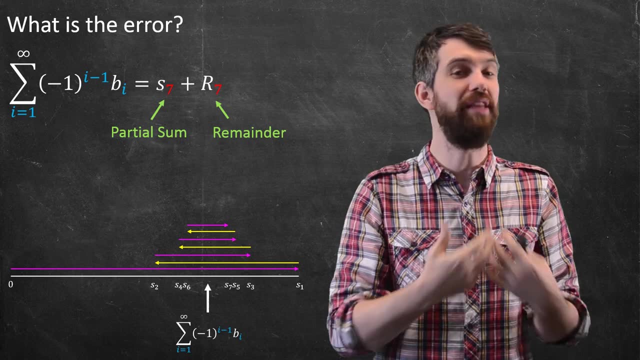 out to the S8, we would then come back to an S9 and go out to an S10 and so on. But based on the way that this collapsing works is the furthest I can ever get away from S7 in the entire rest of. 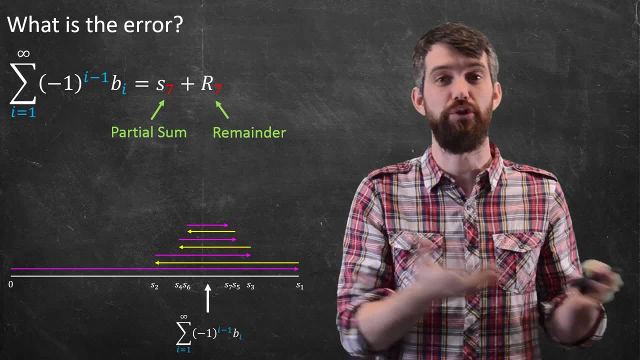 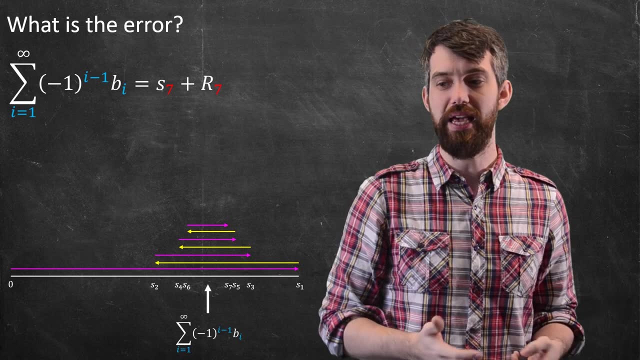 the series is going to go to S8. Because after that I'm going to get closer and closer and closer. That's the way this alternative works. So, whatever the remainder is, I can definitely say that that R7 is going to be less than the. 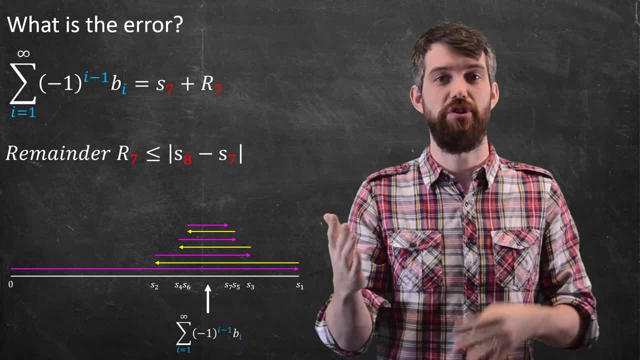 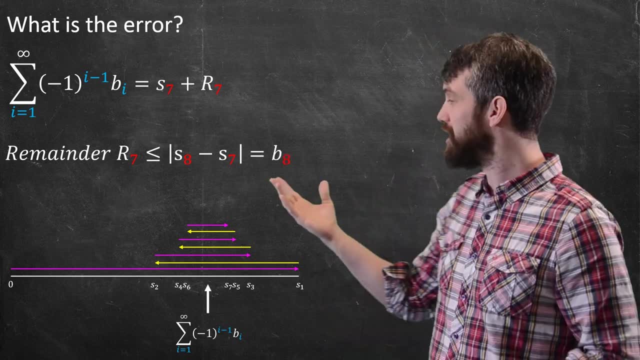 distance between S8 and S7. That is, between the one term and the next one, And indeed the difference between S7 and S8 is just whether I've added the eighth term on, As in this is just that B8. So, in other words, my R7, my remainder, when I take seven terms. 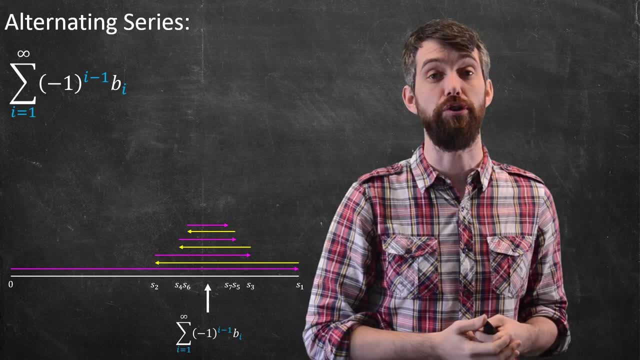 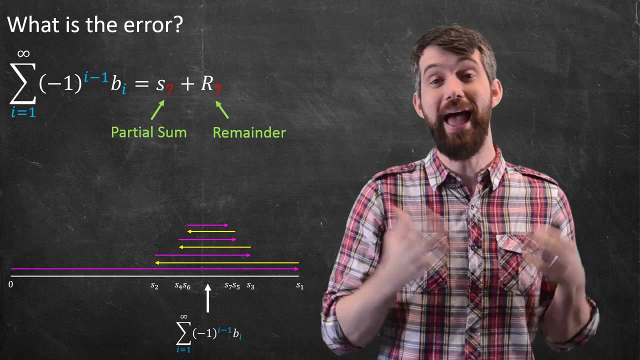 and try to estimate this by perhaps only these first seven terms. That is, I have this series and I want to assume that the sum of the series is going to converge in this kind of case, want to go and write it as the sum of a partial sum- S7, and some remainder, some error term, R7. 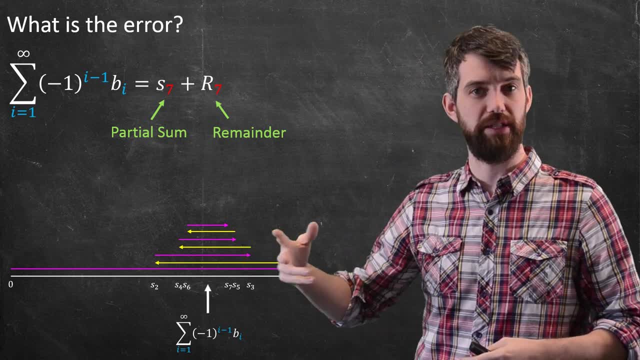 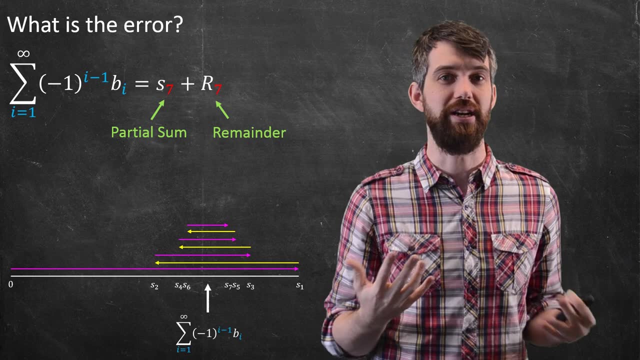 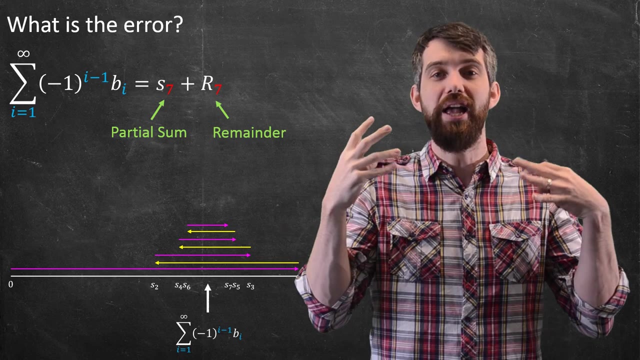 Now I don't know where exactly this sum is. It could be anywhere in this particular region, But let me try to approximate it by, say, the S7.. So the question is: how good is this error? If I take this R7, is it a small number? Is it a big number? How can I control how bad my estimate? 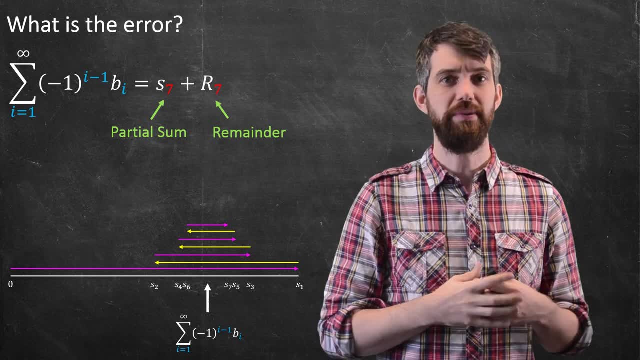 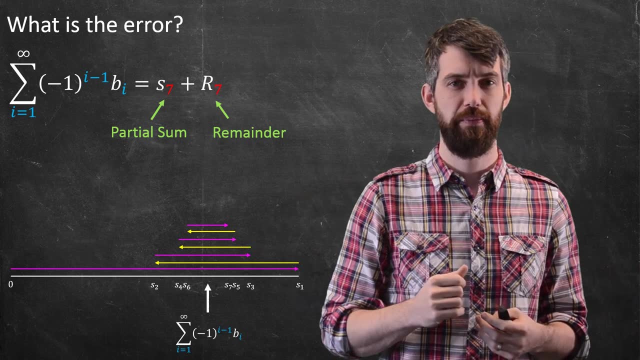 of only taking the first seven terms is going to be Now to think about what this remainder could be. we're currently at the S7. And imagine we want to go from the S7 out to an S8. Well, after we went, 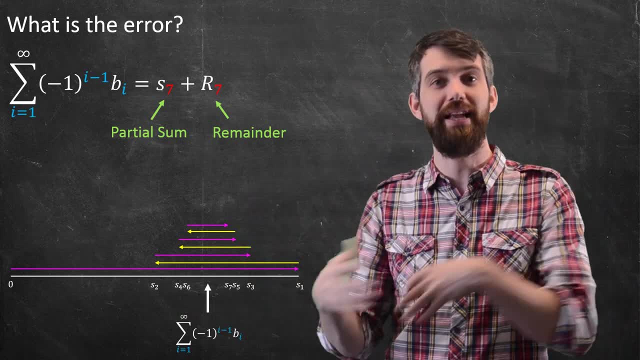 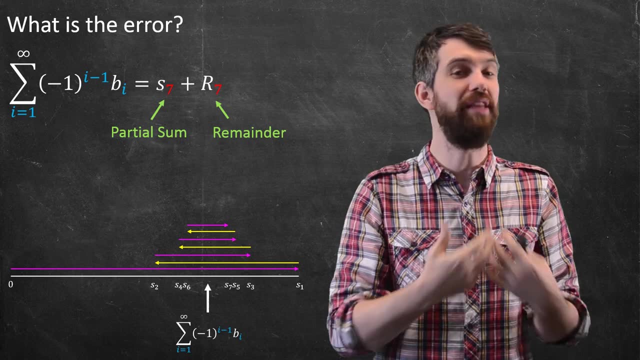 out to the S8, we would then come back to an S9 and go out to an S10 and so on. But based on the way that this collapsing works is the furthest I can ever get away from S7 in the entire rest of. 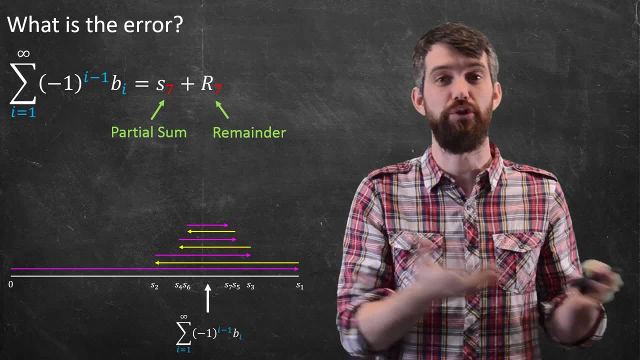 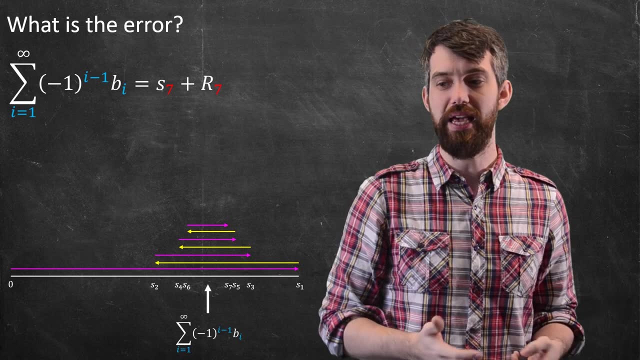 the series is going to go to S8. Because after that I'm going to get closer and closer and closer. That's the way this alternative works. So, whatever the remainder is, I can definitely say that that R7 is going to be less than the. 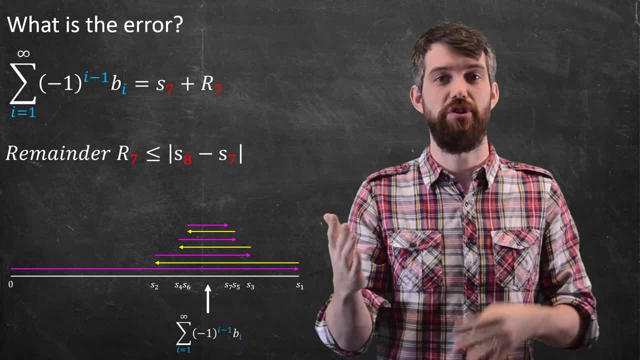 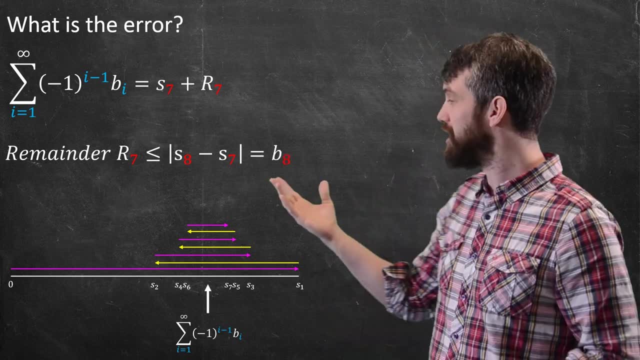 distance between S8 and S7. That is, between the one term and the next one, And indeed the difference between S7 and S8 is just whether I've added the eighth term on, As in this is just that B8. So, in other words, my R7, my remainder, when I take seven terms. 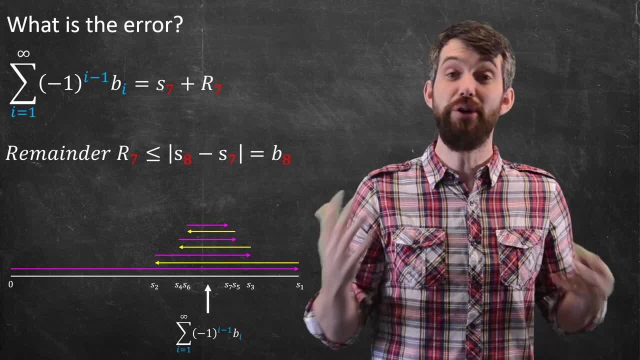 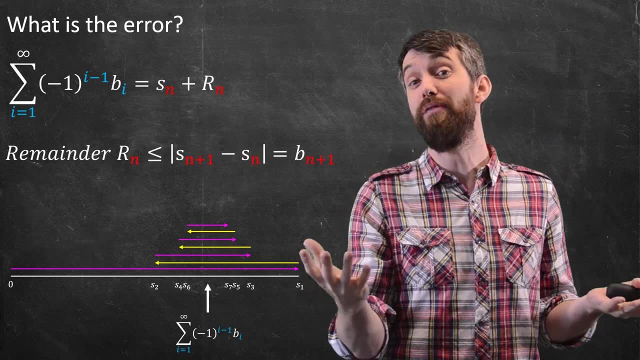 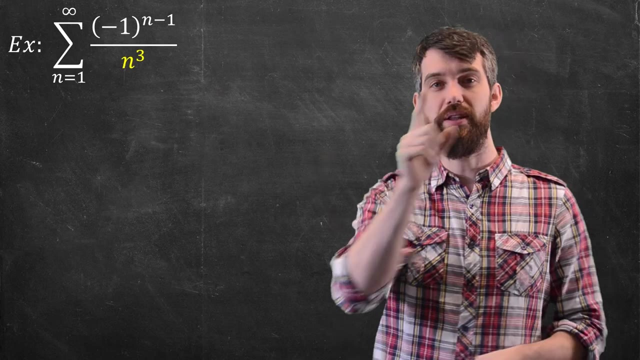 is just bounded by whatever the eighth term is, And in general, if I replace seven here with N, I can say that my remainder of N terms is just going to be whatever the N plus one term was. So let's see how this works out in a specific example. So I've got minus one to the N minus. 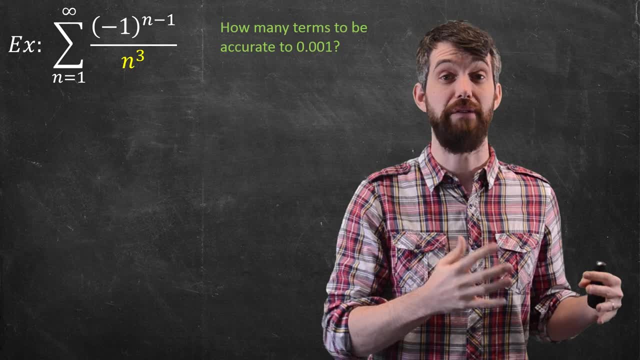 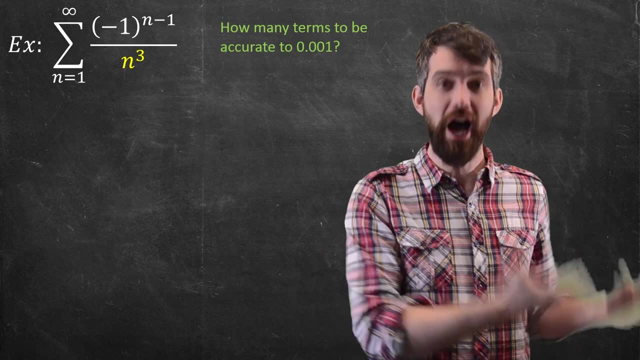 one divided by N, cubed here. And then I'm going to say that for my application, I'm interested in accuracy of 0.001.. Now, how can I ensure that I have enough terms to get that accuracy? Well, if I look at where my remainder is going to be, if I want to estimate, 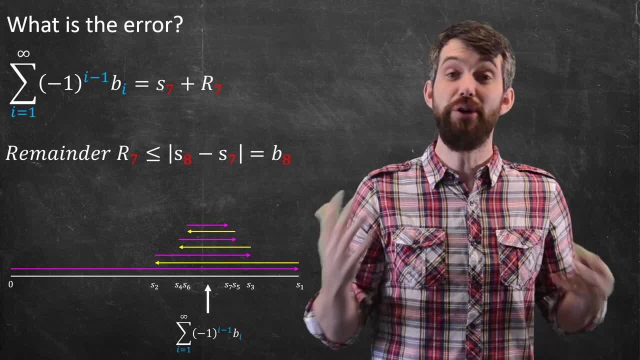 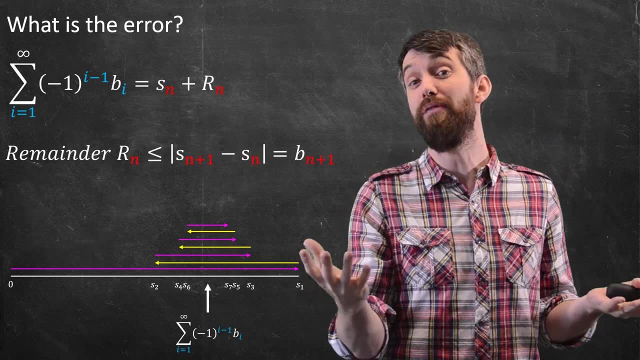 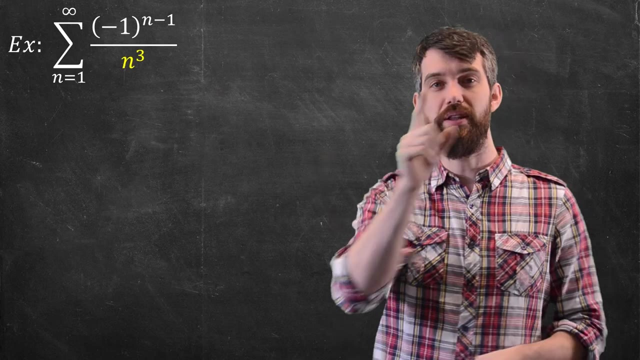 is just bounded by whatever the eighth term is, And in general, if I replace seven here with N, I can say that my remainder of N terms is just going to be whatever the N plus one term was. So let's see how this works out in a specific example. So I've got minus one to the N minus. 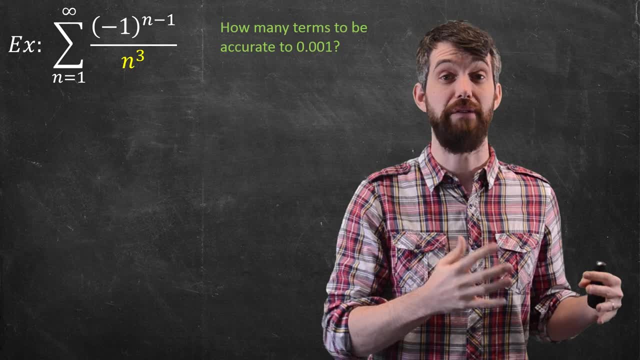 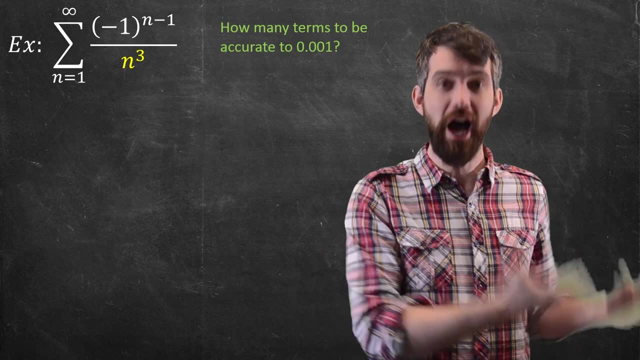 one divided by N, cubed here. And then I'm going to say that for my application, I'm interested in accuracy of 0.001.. Now, how can I ensure that I have enough terms to get that accuracy? Well, if I look at where my remainder is going to be, if I want to estimate, 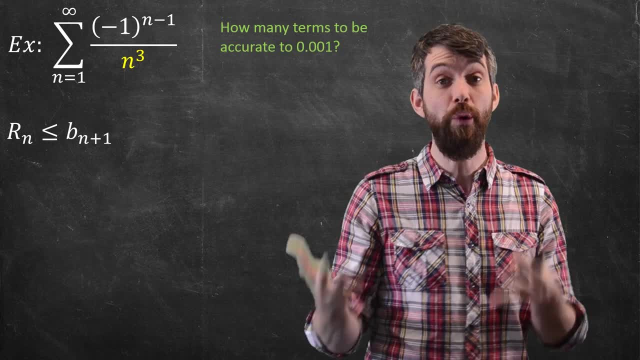 what Rn was. I'm going to say that Rn is going to be 0.001.. And then I'm going to say that Rn is. what we've just seen is that I can bound that by the N plus one term. What I want, this N plus one. 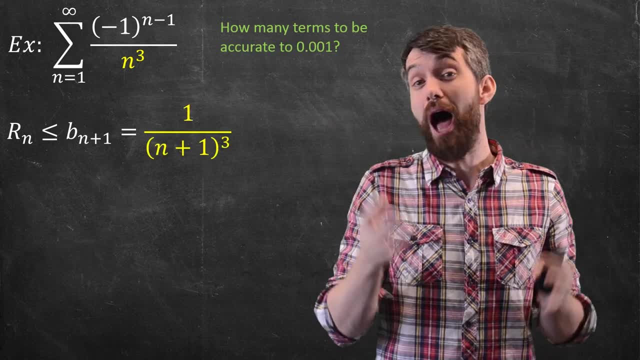 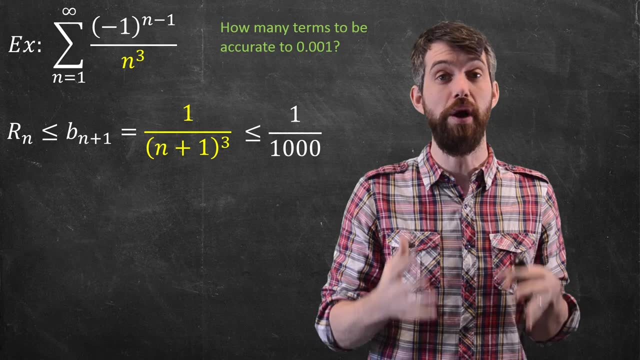 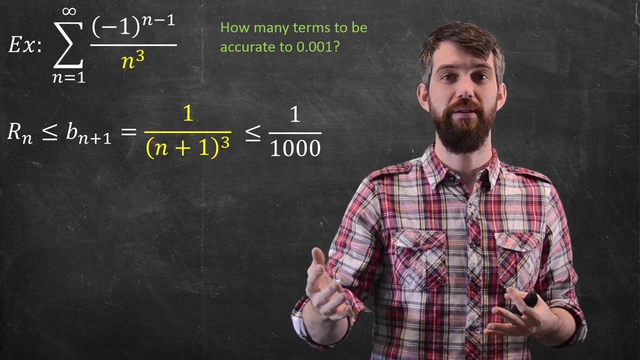 term to be, and it is just remember, one over N plus one cubed. I want that to be less than this 0.001.. So now I have this relationship here, that the one over N plus one cubed needs to be less than one over 1000, which is another way of saying 0.001.. Okay, this is an inequality, So I can just. 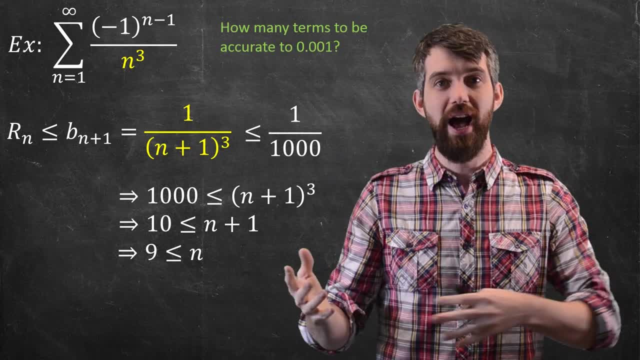 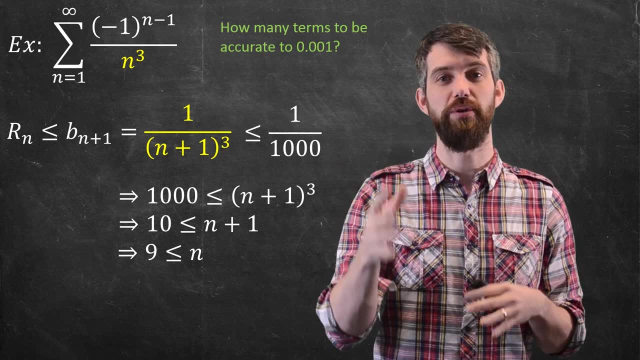 multiply it up, That's: 1000 is less than N plus one. I can take the cube root of both sides, I can get 10 is less than N plus one And finally I can say that N is less than or equal to N. So what does this tell me? It tells me that as long as I take 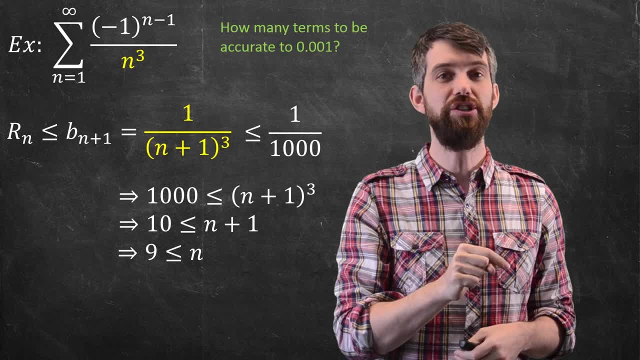 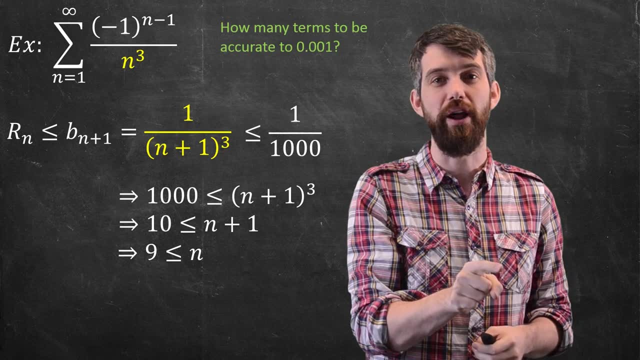 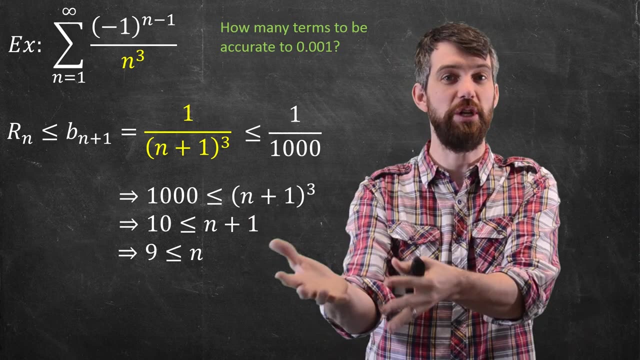 N as nine or bigger, then that ensures that whatever approximation I write out my ninth partial sum, then that ninth partial sum will be accurate to within 0.001.. Now the final point to make here is that in whatever application you may actually be doing this, you're going to be 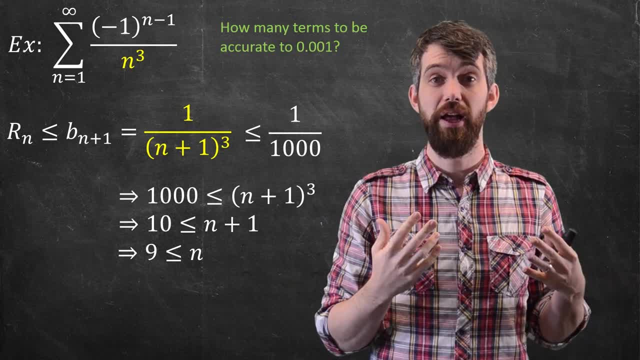 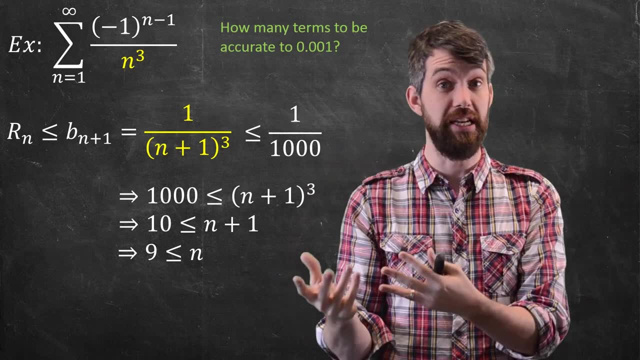 doing in your future careers, whether it's some engineering application or otherwise. there's going to be an uncertainty that comes from that different discipline, And the idea here is this is: it doesn't matter what the uncertainty is to calculus If you come in with the restriction. 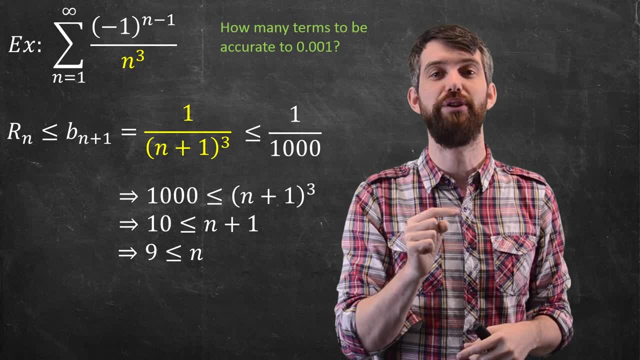 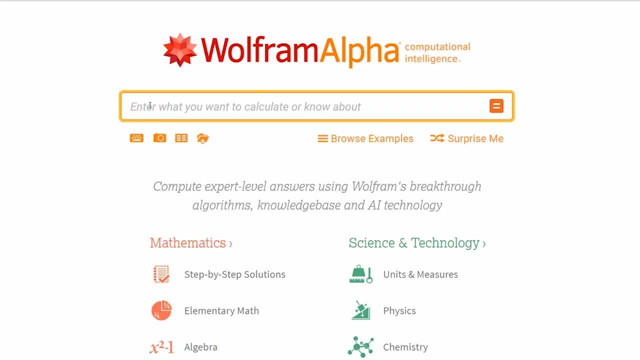 you need it to be however certain you want. You can use this to figure out how many terms you need to get that desired level of certainty. Going back to wolfromelvacom, let's go and try to compute out a few things. I'm going to take the sum of the particular series, which was the. 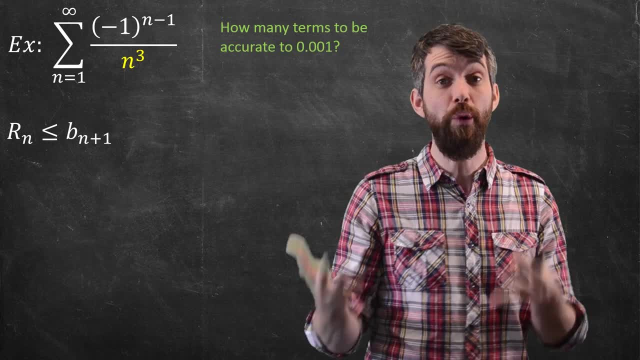 what Rn was, I can say that my remainder of N terms is going to be 0.001.. And then I'm going to. what we've just seen is that I can bound that by the N plus one term. What I want, this N plus one. 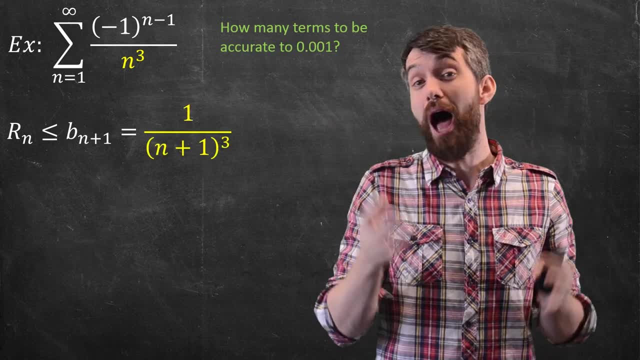 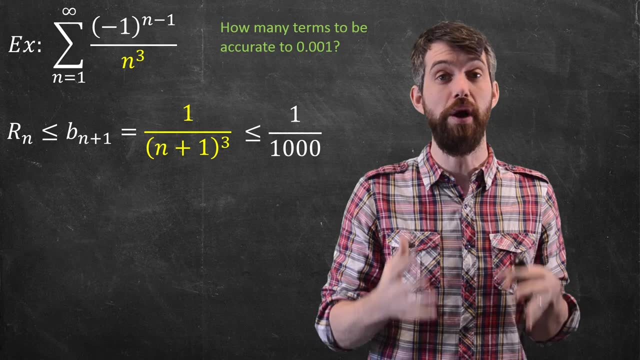 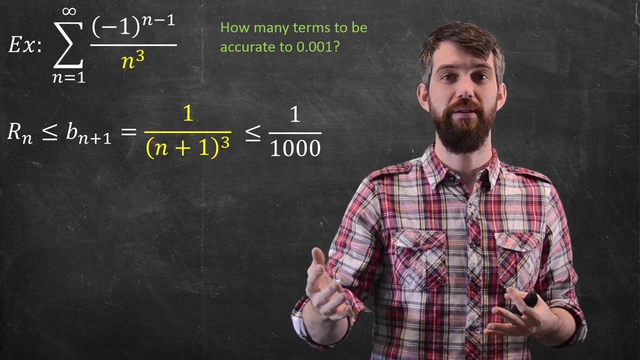 term to be, and it is just remember, one over N plus one cubed. I want that to be less than this 0.001.. So now I have this relationship here, that the one over N plus one cubed needs to be less than one over 1000, which is another way of saying 0.001.. Okay, this is an inequality, So I can just. 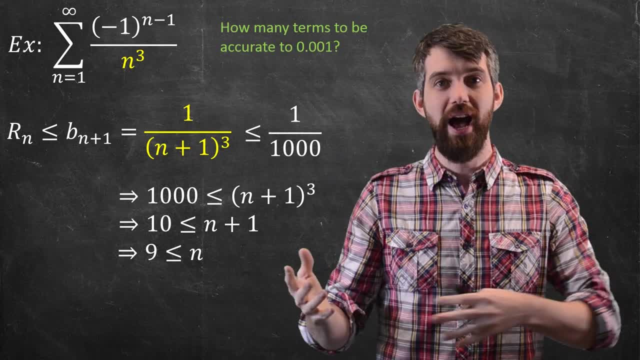 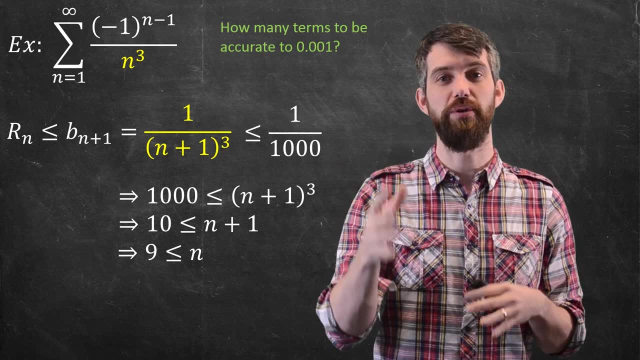 multiply it up, That's: 1000 is less than N plus one. I can take the cube root of both sides, I can get 10 is less than N plus one And finally I can say that N is less than or equal to N. So what does this tell me? It tells me that as long as I take 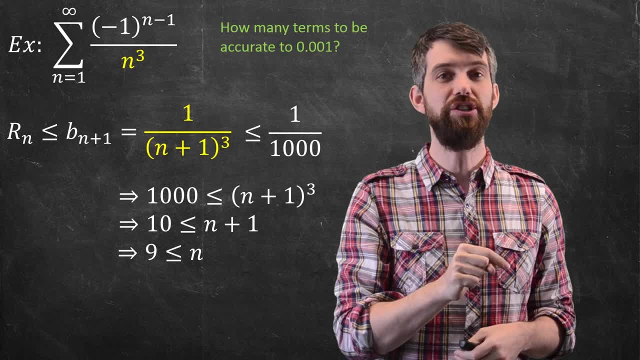 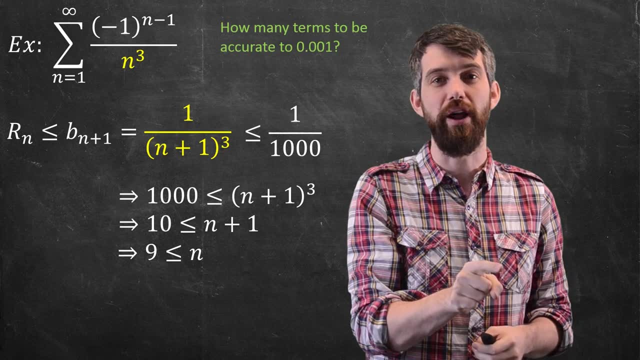 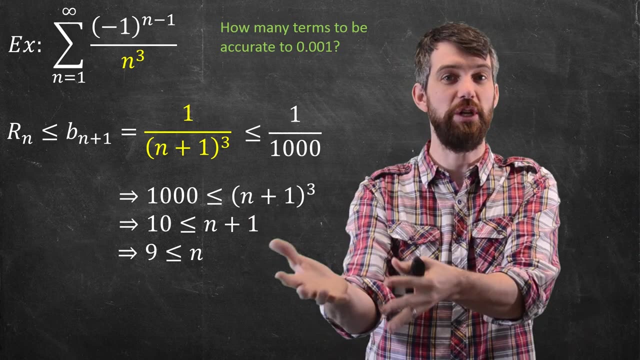 N as nine or bigger, then that ensures that whatever approximation I write out my ninth partial sum, then that ninth partial sum will be accurate to within 0.001.. Now the final point to make here is that in whatever application you may actually be doing this, you're going to be 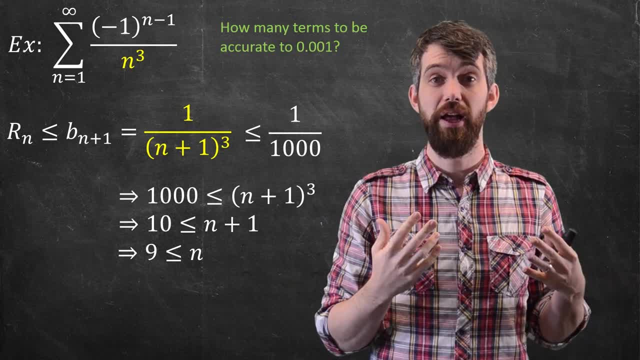 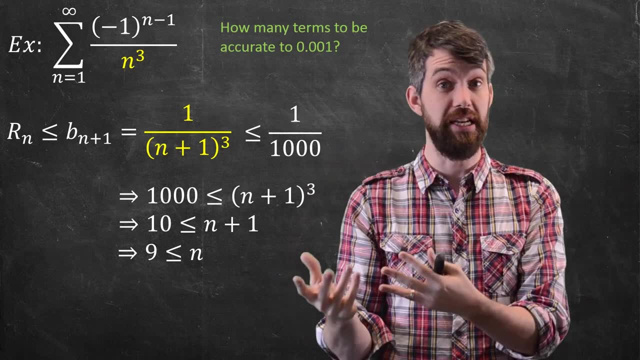 doing in your future careers, whether it's some engineering application or otherwise. there's going to be an uncertainty that comes from that different discipline, And the idea here is this is: it doesn't matter what the uncertainty is to calculus If you come in with the restriction. 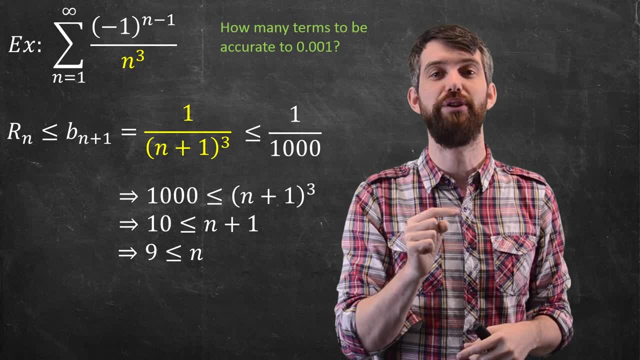 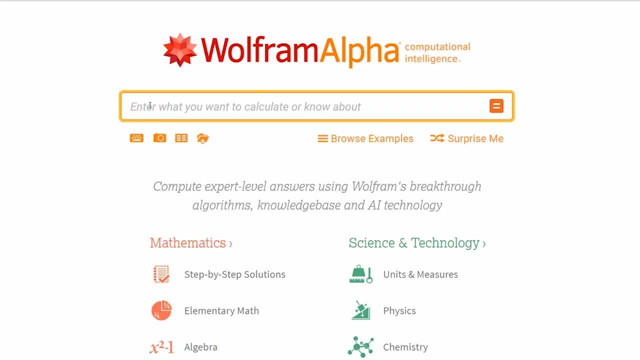 you need it to be however certain you want. You can use this to figure out how many terms you need to get that desired level of certainty. Going back to wolfromelvacom, let's go and try to compute out a few things. I'm going to take the sum of the particular series, which was the. 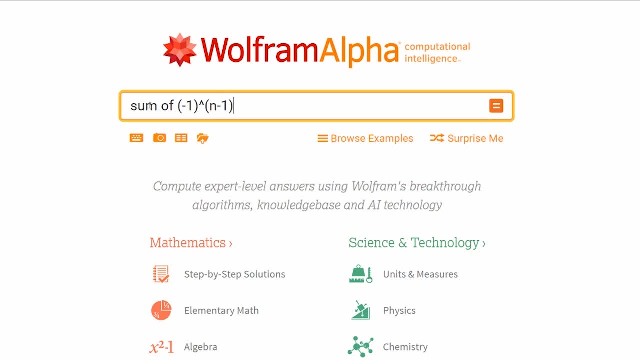 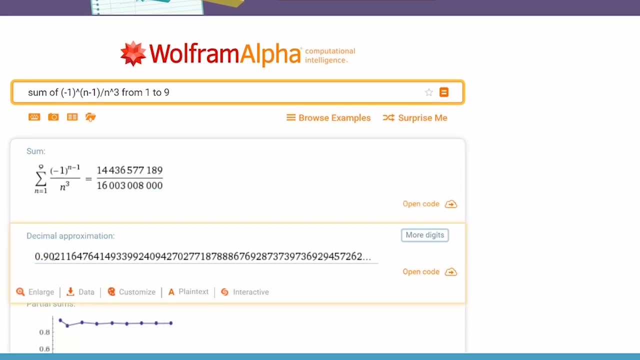 minus one to the power of N minus one, and then all divided by N cubed, And what we want to do is take the approximation from one to nine, because nine told us how many terms we're going to need. So I do that computation And what do I get? it looks like a value of 0.902.. Now, this is only. 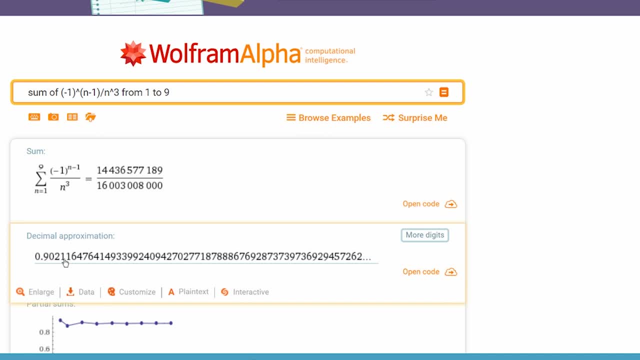 taking nine terms, And what we guaranteed is that we are within point 001 of the correct answer if I took the N minus one to the power of N minus one And what we want to do is take the approximation as many terms as I could possibly want, And indeed let me just try just for fun here How 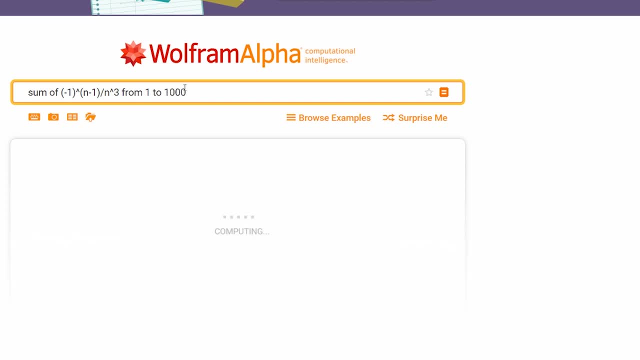 about instead of one to nine. I just put in 1000 terms, So this is going to be a huge number of terms. it's going to take a little while for it to compute. And there it goes. So it says that if 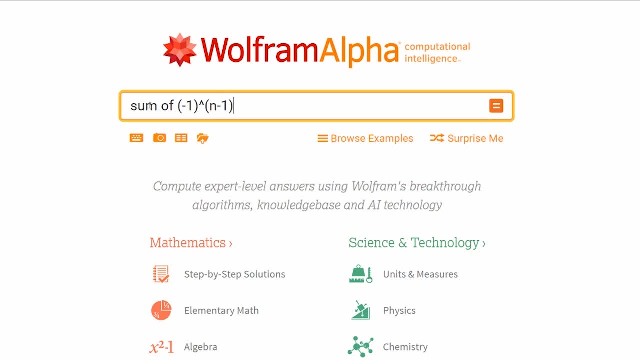 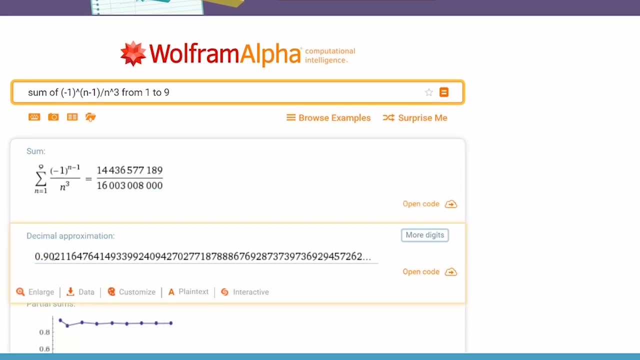 minus one to the power of N minus one, and then all divided by N cubed, And what we want to do is take the approximation from one to nine, because nine told us how many terms we're going to need. So I do that computation And what do I get? it looks like a value of 0.902.. Now, this is only.